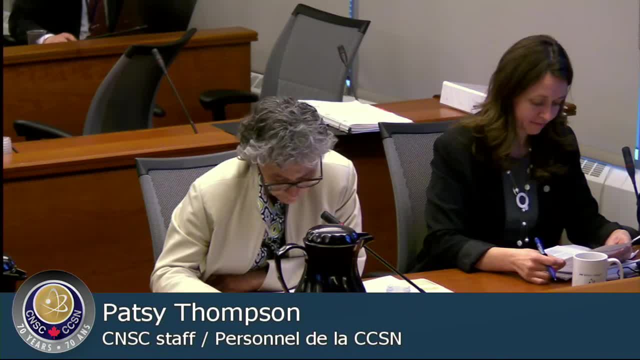 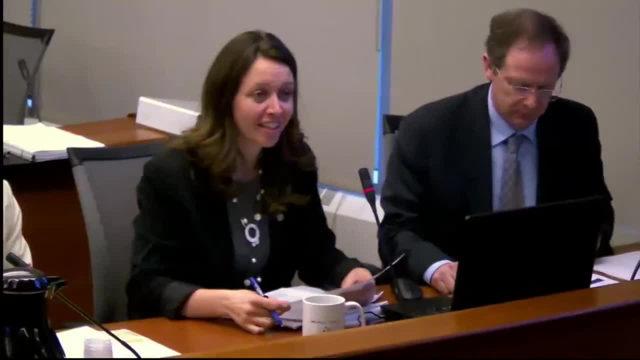 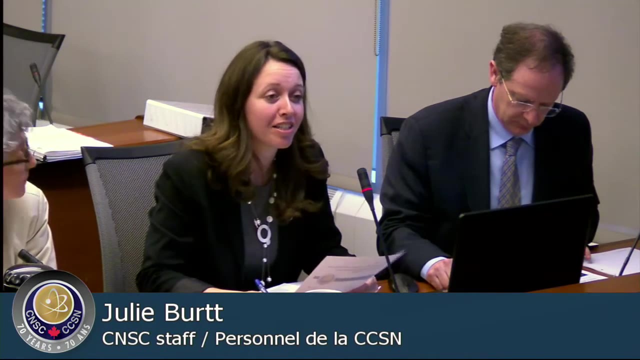 for radiation protection of workers and members of the public. I will ask Ms Burt to make the staff's presentation. Thank you, Dr Thompson. My name is Julie Burt. As mentioned, I am a Radiation and Health Sciences Officer with expertise in the exciting field of radiation biology. Before we begin, 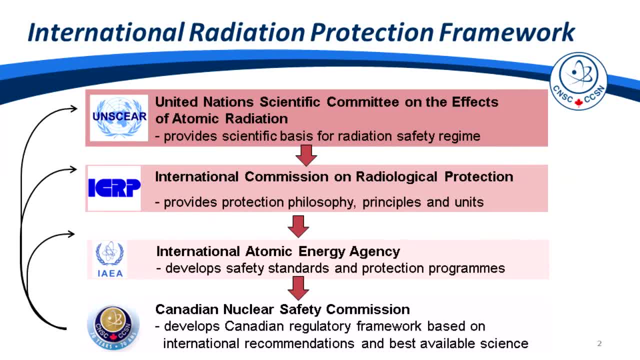 I'd like to take the time to highlight the main international agencies who contribute to the Radiation Protection Regulatory Framework, as I will be discussing their role and scientific position on certain matters throughout today's presentation. First off, the United Nations Scientific Committee on the Effects of Atomic Radiation. 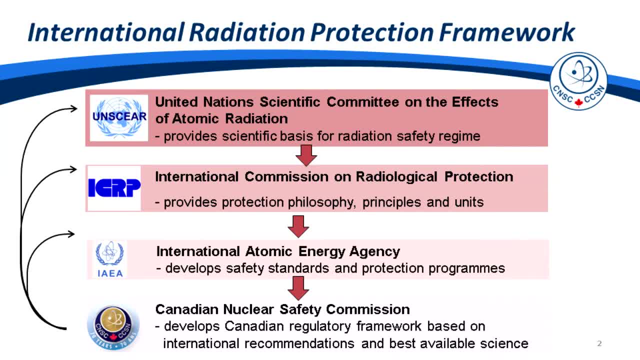 or UNSCEAR, provides the scientific basis for the radiation safety regime. Secondly, the International Commission on Radiological Protection, or ICRP, takes the information from UNSCEAR, the international scientific literature and socio-economic factors and provides protection, philosophy, principles and units. We often refer to these collectively. 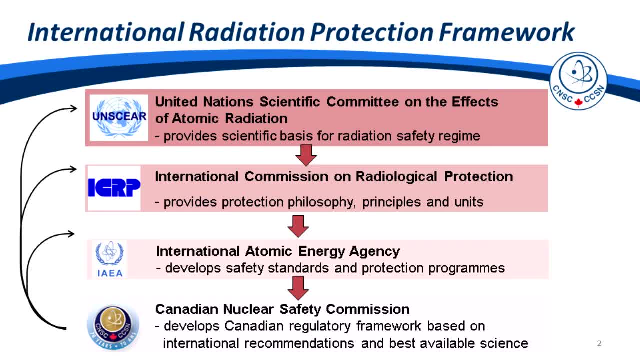 as the ICRP recommendations. Next, the International Atomic Energy Agency, or IAEA, develops safety standards and protection programs for member states to adopt. Finally, the Canadian Nuclear Safety Commission, or CNSC, uses all of this information to develop Canada's regulatory framework, which is based 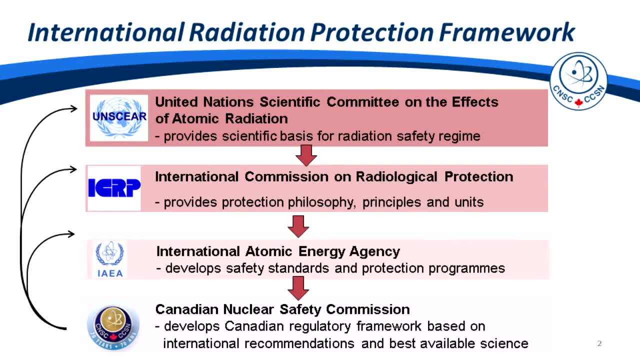 on the best available science. Perhaps the most critical part of this figure is that CNSC's staff provide expertise to all of these international agencies – whether it be from staff serving as delegates or delegates sitting on working groups or providing comments on draft publications. 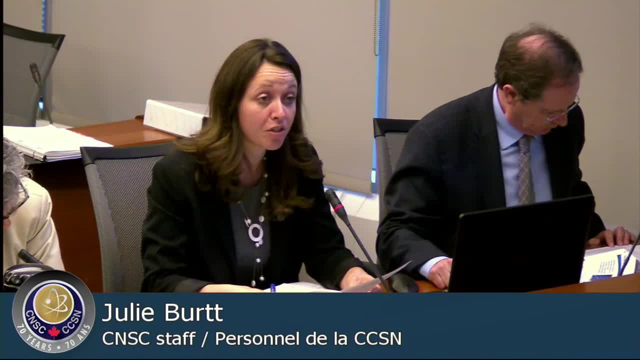 CNSC staff are very involved when it comes to shaping the international regulatory framework. Furthermore, the CNSC can deviate from international guidance and recommendations to ensure Canada's best interests are being met. Similarly, other countries have developed their framework based on what is best for. 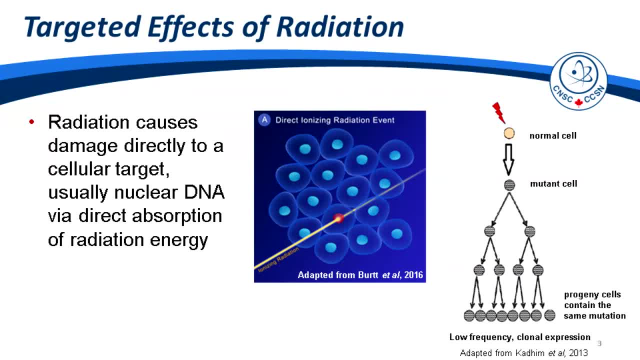 their country Historically the best available. science has taught us that, according to the classic target theory of ionizing radiation, deleterious effects such as mutations or cancer are attributed to radiation damage to a cellular target usually identified as nuclear DNA. This occurs due to the direct absorption of radiation energy, the consequences of which 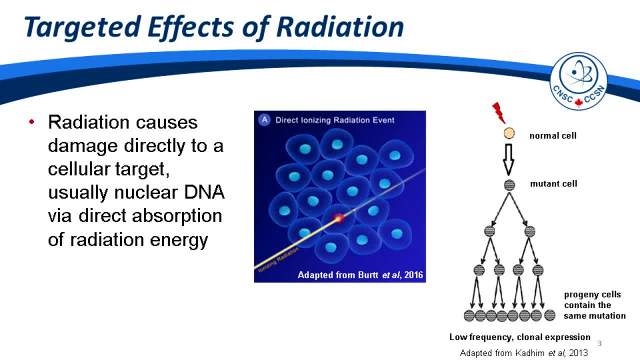 are expressed in the surviving irradiated cells. The image on the left shows ionizing radiation. The image on the right shows ionizing radiation passing through the nucleus of one cell and only damaging that nucleus. The image on the right shows a normal cell being hit by radiation, creating a mutation. 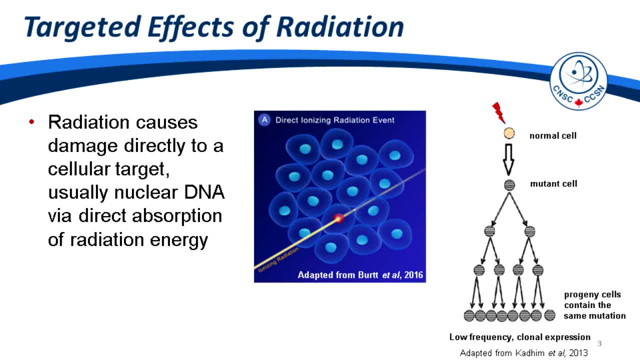 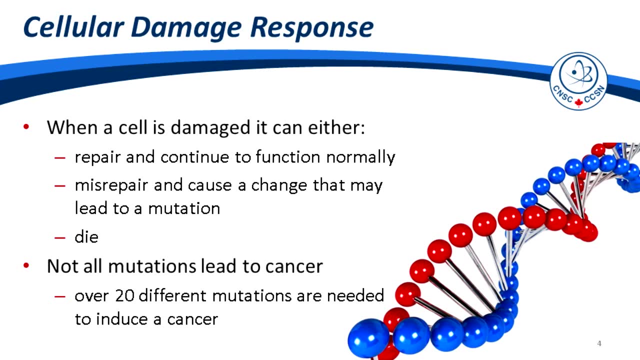 That same mutation is passed on to progeny or daughter cells after each cell division. These two images are both demonstrating the targeted effects of radiation. However, most of the time when radiation causes damage, it is not only the cell that is damaged. 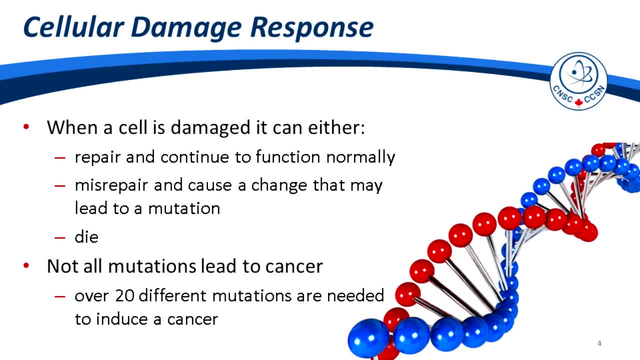 the cell dies or is repaired. Very rarely the cell is not repaired properly and possibly leads to a mutation. It's important to note that not all mutations lead to the development of a cancer. In fact, it takes on the order of 20 mutations before a cancer develops. 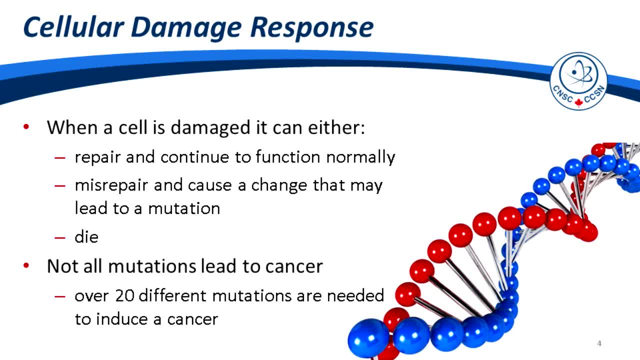 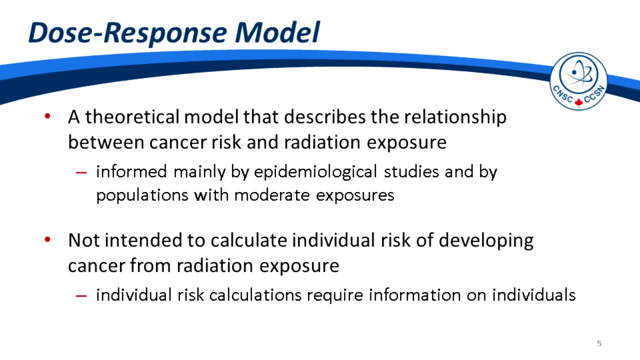 Based on this understanding of how radiation behaves and affects cells, a dose-response model was developed to describe how the risk of cancer varies with radiation dose. A dose-response model is a theoretical model that has been established from what we know about the targeted effects of radiation in populations with moderate exposures. 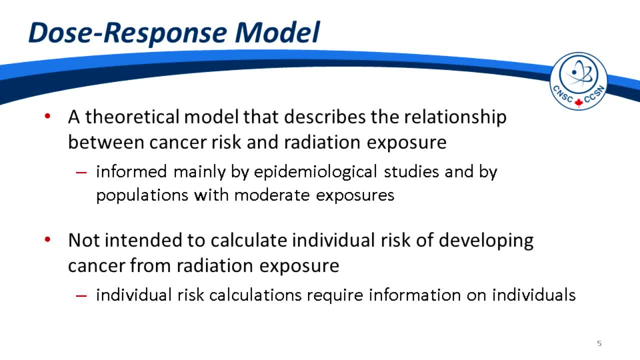 A dose-response model is not intended to calculate individual risk of developing cancer from radiation exposure. An assessment of individual risk requires information on a person's radiation dose, the dose rate, that person's age and sex, as well as other lifestyle, genetic and environmental factors. 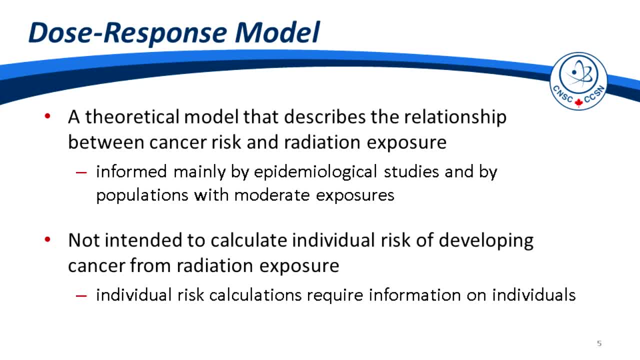 So the venous system is not always a good fit for a cancer. Despite this information, cancer, if it occurs in an individual, cannot unequivocally be attributed to radiation exposure, because radiation exposure is not the only possible cause And there are no generally available biomarkers that are specific to radiation-induced effects. 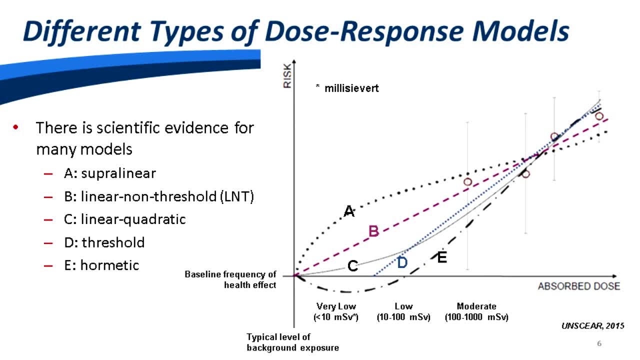 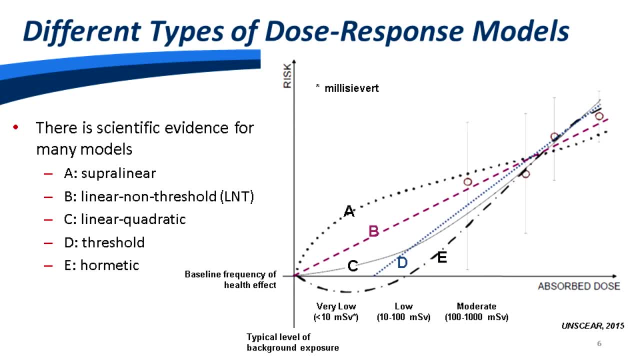 The x- and y-axis meet at the baseline risk of a health effect. So everything shown on this graph is on top of the natural risk level of developing cancer. In Canada, the baseline risk of developing cancer is between 40 and 45 percent. 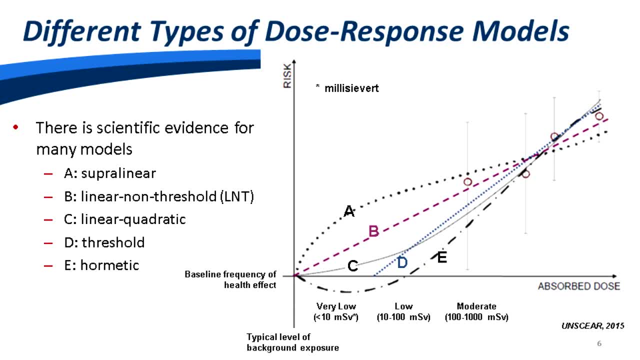 The data points on the graph are shown as open circles with vertical uncertainty bars. These data points come directly from epidemiological studies, for which sound data becomes available at approximately 100 millisieverts. Error bars for each data point demonstrate the wide range of data used to establish the 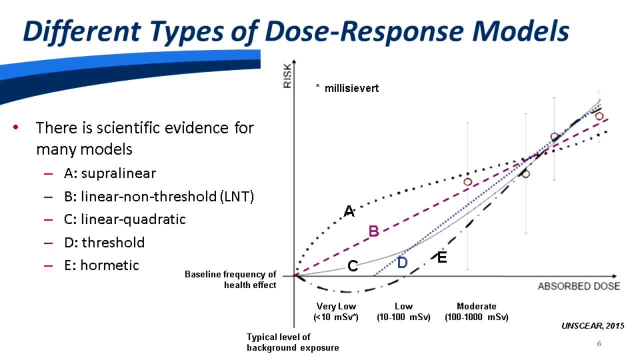 average data point. The lowest dose at which excess cancers or cancers caused by radiation and not some other factor have been observed in adult populations is approximately 100 millisieverts. The different lines on the graph show. the different lines on the graph show: 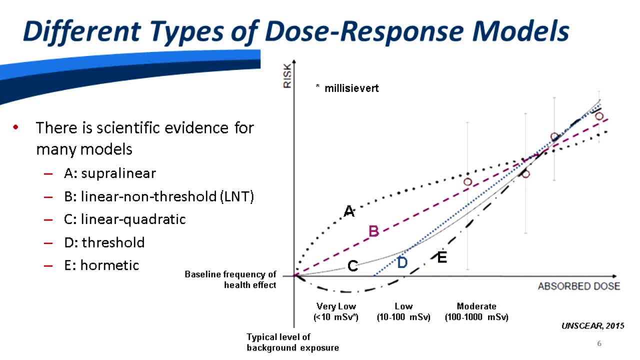 possible radiobiological mechanisms acting at low doses. The regulatory dose-response model currently used to describe how cancer risk varies with radiation dose is called the Linear Non-Threshold Model, or LNT for short, shown here as line B. The LNT model assumes that harmful effects occur in directly hit or targeted cells. 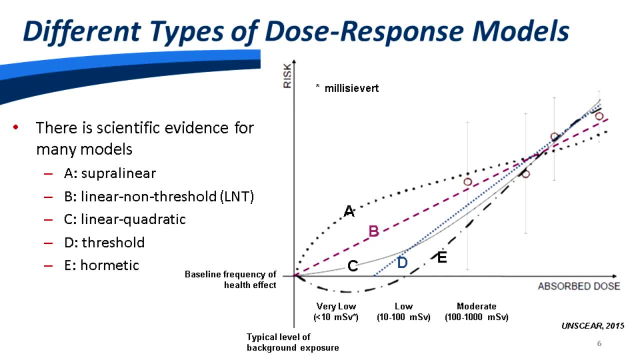 and the risk from developing cancer from these effects increases as the dose increases. Most types of cancer can be treated with radiation. There is also strong scientific evidence for other types of dose-response models. Line A is super-linear. This model suggests that there is a greater risk of developing cancer at lower doses. 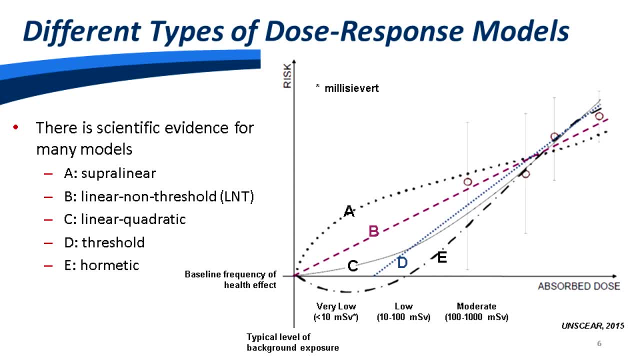 Line C is linear-quadratic. This model suggests that repair mechanisms may be more effective at very low and low doses than at higher doses, For example. this is the model adopted internationally. This model is used internationally to estimate the risk of leukemia. Line D has a threshold. 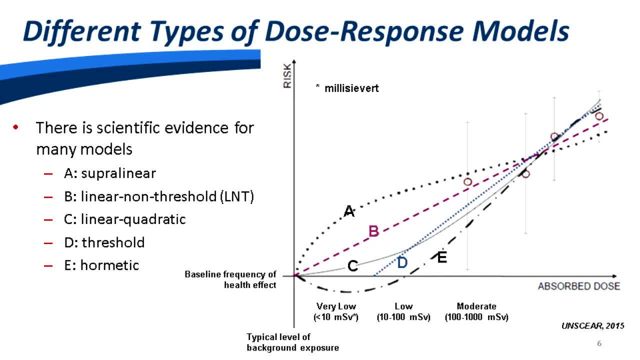 This model suggests that below a certain dose there is no risk. For example, this is the case for bone cancer from exposure to radium-226.. Line E shows the hormesis model, which suggests that exposure to low doses induces a protective or beneficial effect. 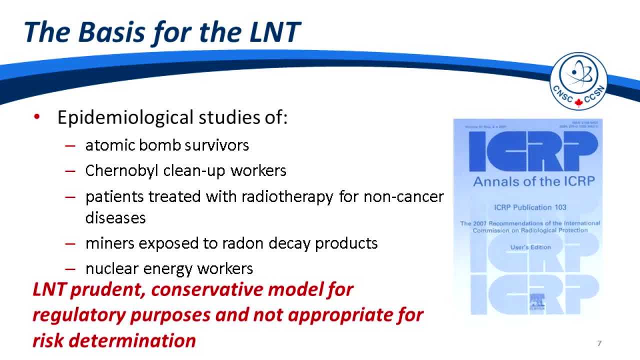 The basis for the LNT model comes from epidemiology. The epidemiological studies which have been found to support the LNT model include the Atomic Bomb Survivor studies, studies of the Chernobyl cleanup workers, studies of patients treated with radiotherapy for non-cancer diseases, studies of miners exposed to radon decay products. 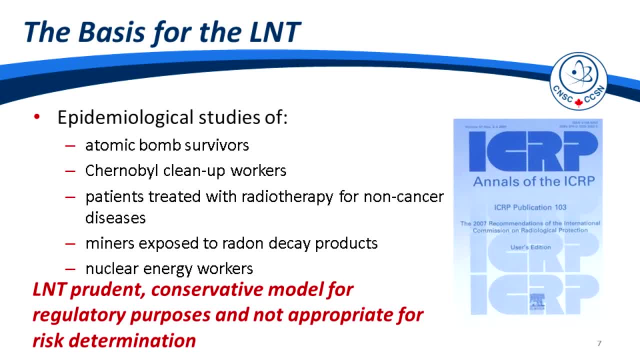 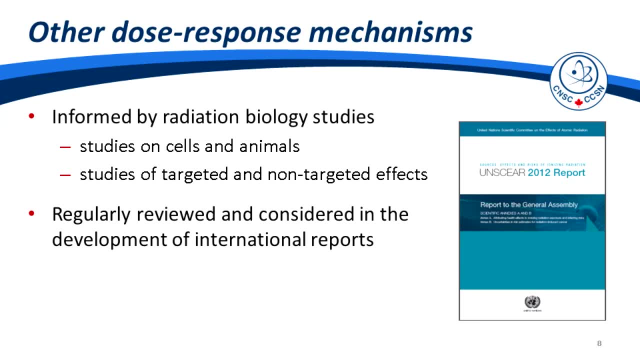 and studies of nuclear energy workers. The LNT model is a prudent, conservative model for regulatory purposes. It is not appropriate for risk determination- Slide 11.. Radiation biology studies refer to studies done on cells or animals. They are used to inform dose response models when no sound epidemiological data is available. 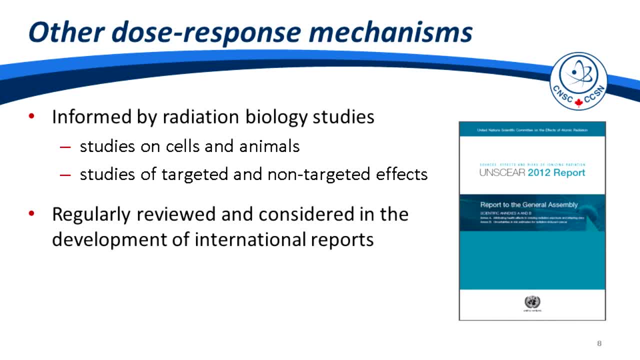 in the low and very low dose region. Both epidemiological and radiation biology studies are reviewed and considered in the development of international reports like those of UNSCEAR and the ICRP. Slide 12.. Slide 13.. Slide 14.. 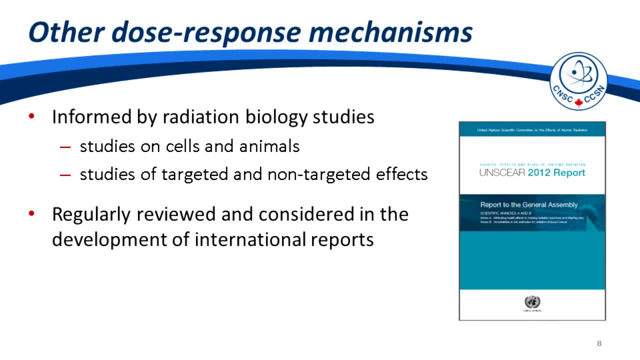 Slide 15.. Slide 16., Slide 17., Slide 18., Slide 19., Slide 20.. Slide 21. Slide 22., Slide 23., Slide 24., Slide 25., Slide 26., Slide 27.. 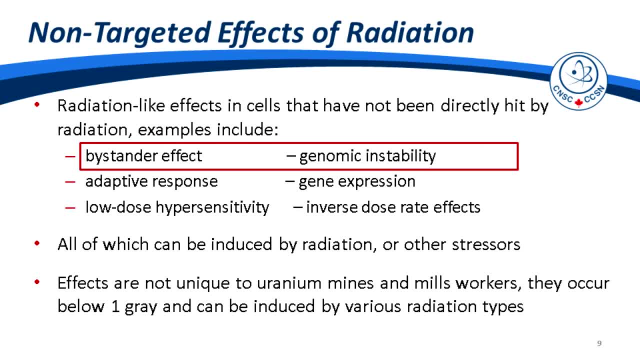 Slide 28.. Slide 29.. Slide 30.. Slide 31.. Slide 32.. Slide 33.. Slide 34.. Slide 35.. Slide 36.. Slide 37.. Slide 38.. Slide 39.. Slide 40.. 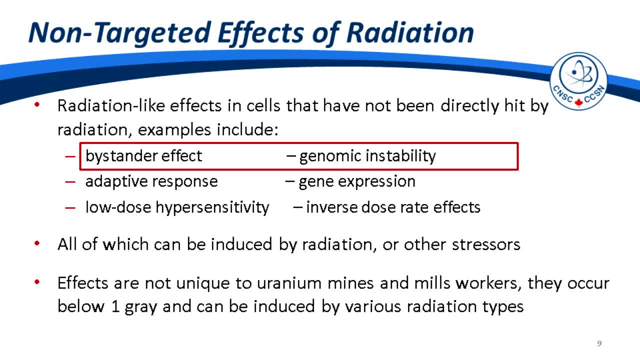 Slide 41., Slide 42., Slide 43., Slide 44., Slide 45., Slide 46., Slide 47., Slide 48., Slide 49., Slide 50., Slide 51., Slide 52.. Slide 53.. 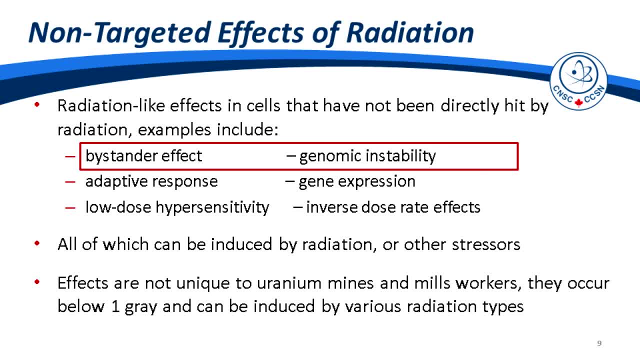 Slide 54. Slide 55.. Slide 56. Slide 56. Slide 57. Slide 58. Slide 58. Slide 59. Slide 59. Slide 60.. Slide 61. Slide 62. Slide 63.. 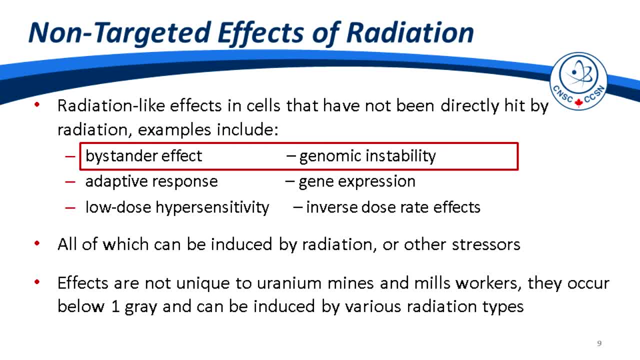 Slide 64.. Slide 65.. Slide 67.. Slide 68.. Slide 69.. Slide 70.. Slide 71.. Slide 72.. Slide 78.. Slide 79.. Slide 80.. Slide 91.. Slide 92.. 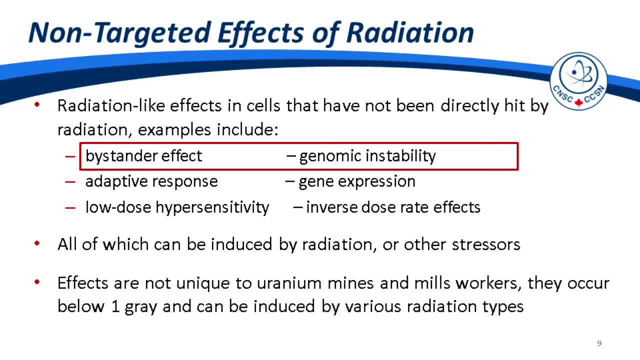 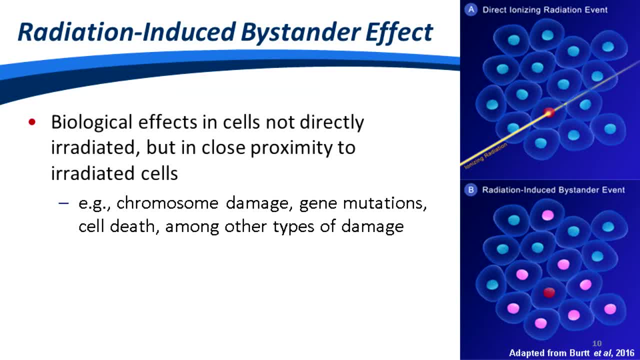 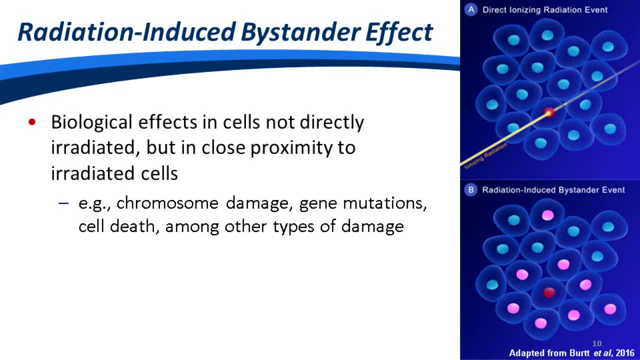 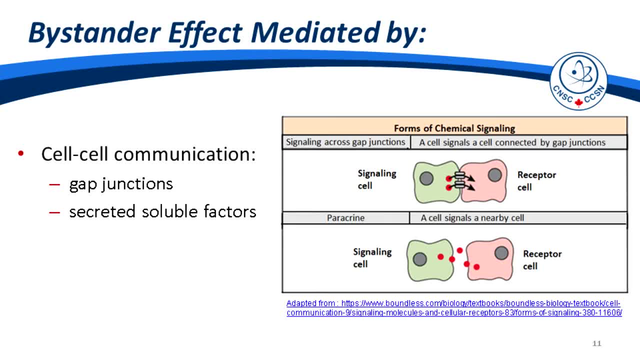 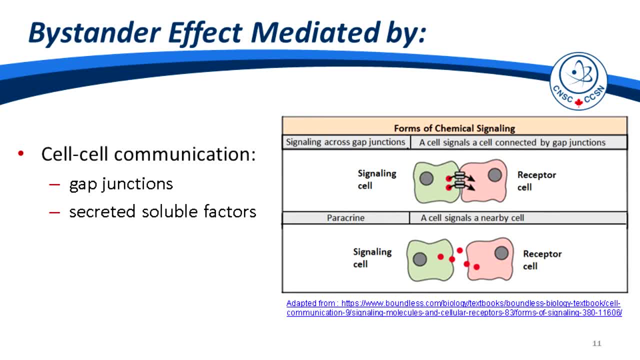 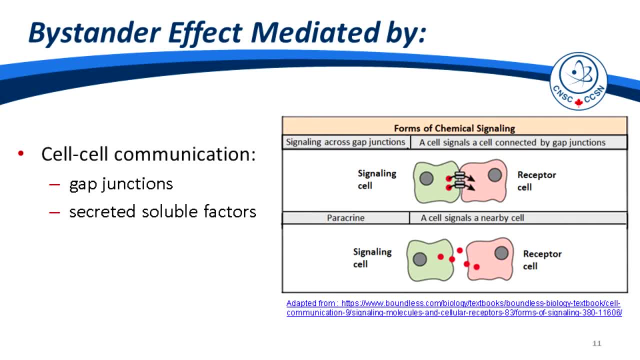 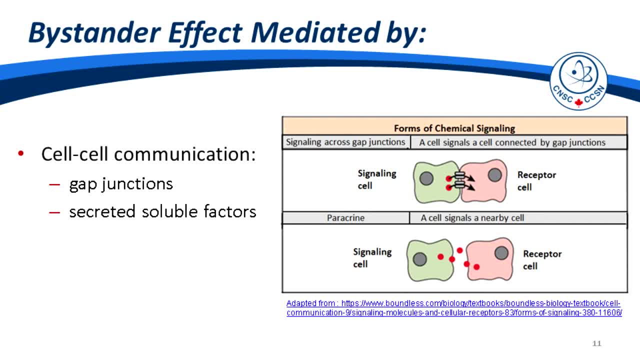 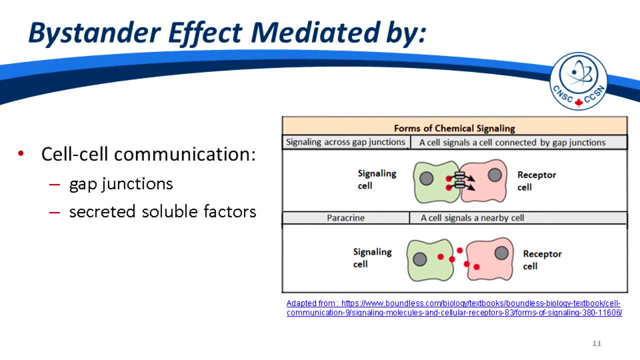 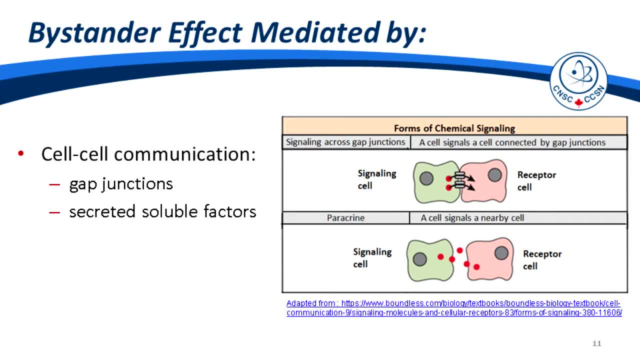 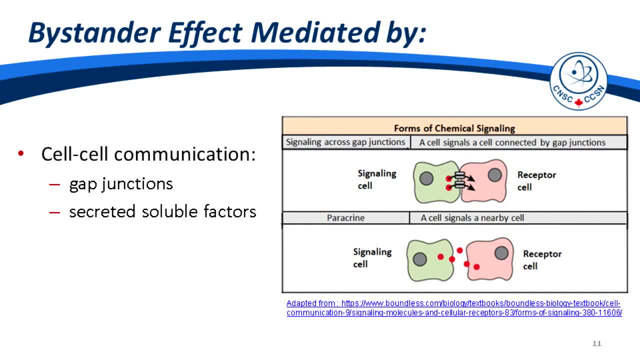 The bystander effect is mediated by two main forms of communication: gap junctions and secreted soluble factors into the extracellular space between cells, As seen in the top picture. gap junction signaling occurs when two cells are right next to each other and their cell membranes may actually be touching. 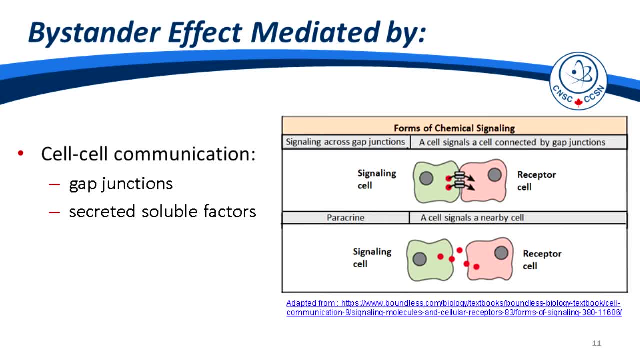 The gap junction is a tunnel-like opening that can allow movement of molecules from one cell to another, As seen in the bottom picture. paracrine signaling occurs when the signaling cell sends molecules that can act locally by diffusing inside other cells that are in the close environment. 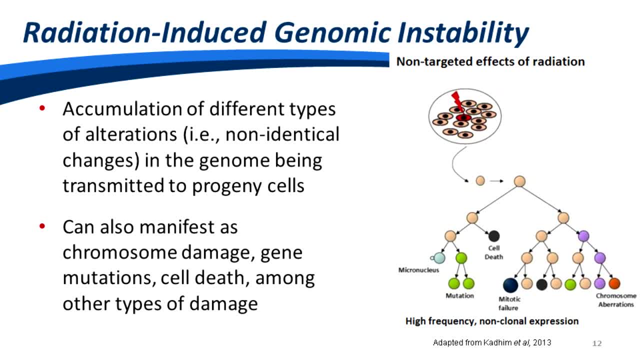 The other non-targeted effect that we are focusing on today is radiation-induced genomic instability. Genomic instability refers to the accumulation of radioactivity. Radiation-induced genomic instability refers to the accumulation of radioactivity in the cell. The radioactivity of radioactivity in the cell is the result of radiation of different types. 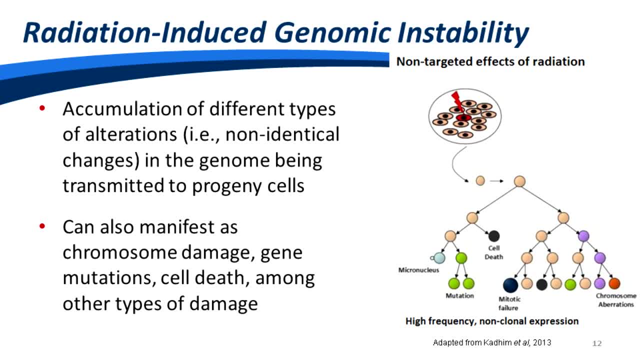 of alterations or changes in the genome being transmitted to progeny or daughter cells. As seen at the top of this figure, the red cell has been directly hit by radiation and the beige cells have not. After cell division, you can see that at different time points the beige cells are turning different. 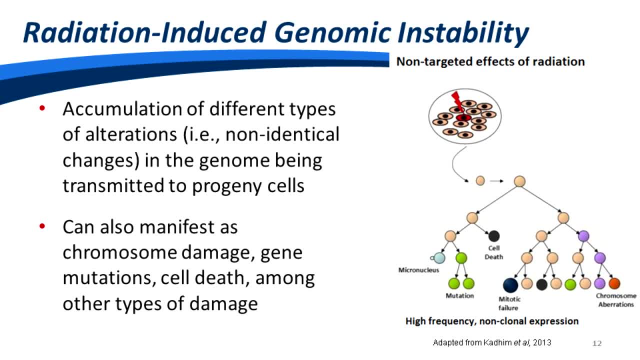 colors representing different forms of damage. The light blue cell has developed a micronucleus, which is a small structure containing genetic material inside the cytoplasm. The green cells have developed a mutation. The black cells have died. The large dark blue cell has failed to go through mitosis or cell division. 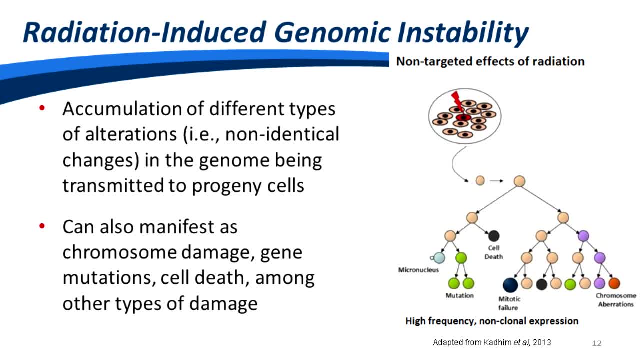 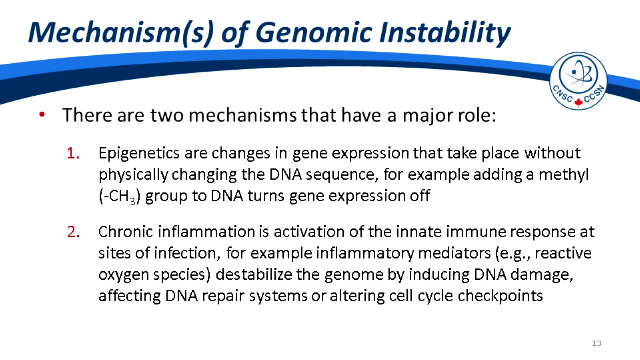 The purple and red cells have suffered changes in the structure or number of chromosomes in the organism. Again, approximately 20 gene mutations are needed before a cell can become carcinogenic. 3. The Detailed Mechanism. The Detailed Mechanism behind genomic instability is not fully understood at this time. What is understood is that epigenetics 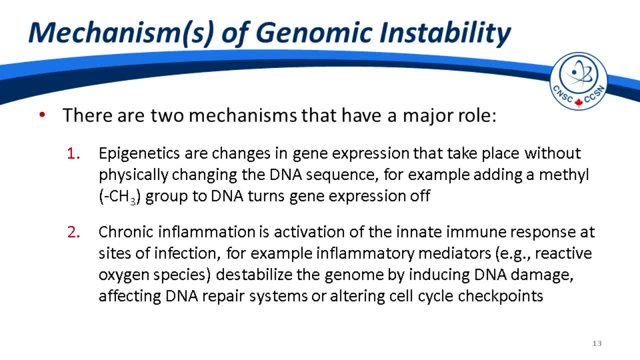 and chronic inflammation play a major role in the perpetuation of genomic instability. Epigenetics are changes in gene expression that take place without physically changing the DNA sequence. An example of this type of change is adding a methyl group, which is a carbon atom. 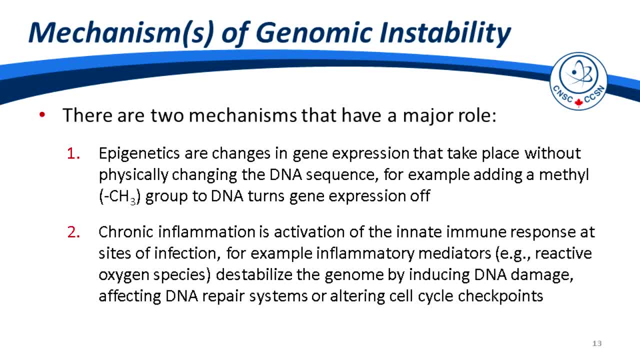 bound to three hydrogen atoms to DNA. Binding this small molecule to DNA has the power to turn gene expression off and effectively stops the gene from doing its job. As part of the immune response, inflammation plays an important role in defending the body against pathogens such as. 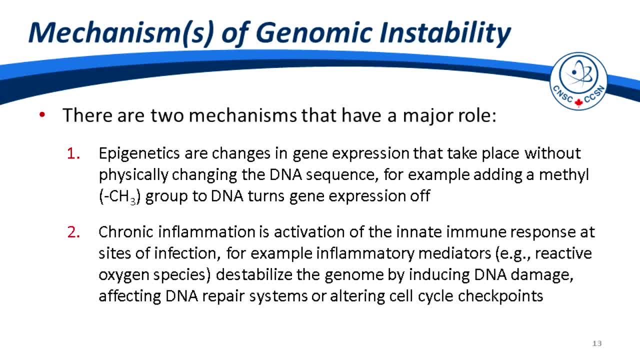 bacteria and viruses. However, inappropriate activation of inflammatory processes is an underlying contributor to many common diseases, including playing a role in tumor proliferation and metastasis. An example of this type of response is the ability of inflammatory mediators like reactive oxygen species, also called 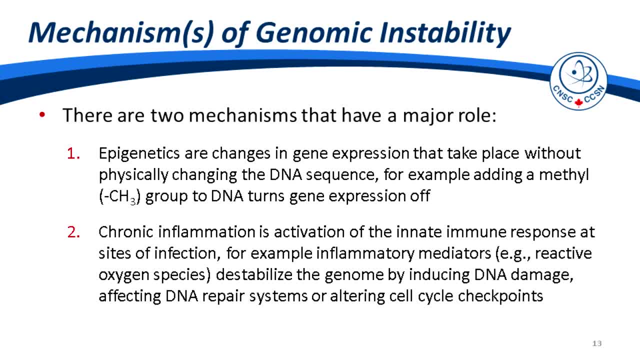 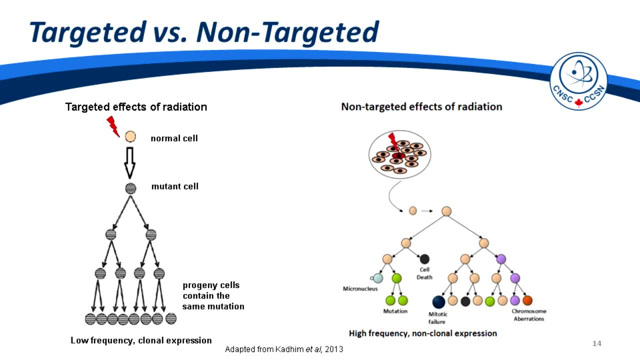 phytoplankton to act as a mediator for inflammatory processes. The other example is the use of cell-free radicals to destabilize the genome by inducing DNA damage or affecting DNA repair systems, or even altering the cell cycle. If we pause here to recap the difference between targeted and non-targeted effects, 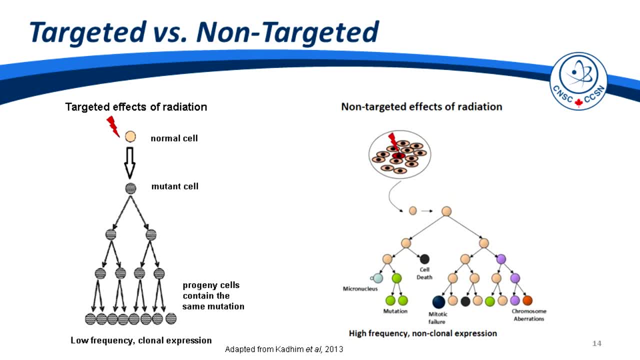 can be shown nicely by putting these two images side-by-side. Targeted effects of radiation are where the progeny cells contain the same mutation as the parent cell, as shown on the left left, and non-targeted effects of radiation are where the progeny cells display different. 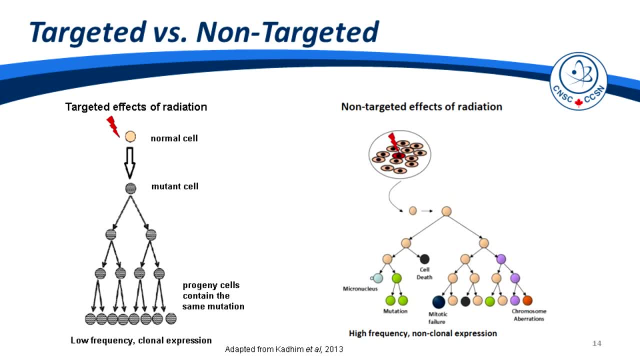 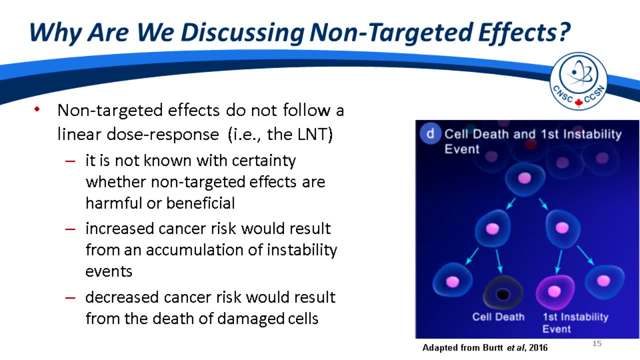 types of damage which were not expressed in the parent cell, as shown on the right. The reason non-targeted effects are important is because they do not follow a linear dose-response curve. It is not known with certainty whether non-targeted effects are harmful or beneficial. 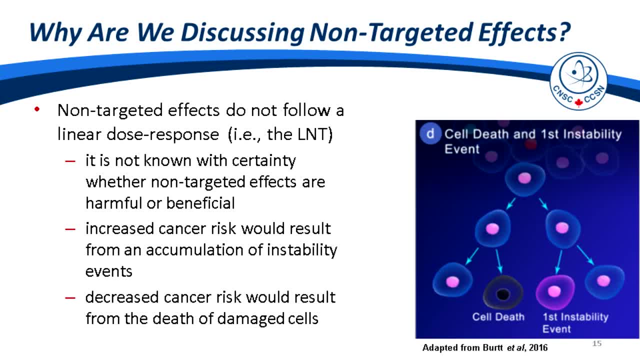 The studies concluding that non-targeted effects could decrease cancer risk are observing high levels of apoptosis or cell death, as shown in black on this figure, A high level of apoptosis results in radiation-induced damage like mutations not being perpetuated during cell division. 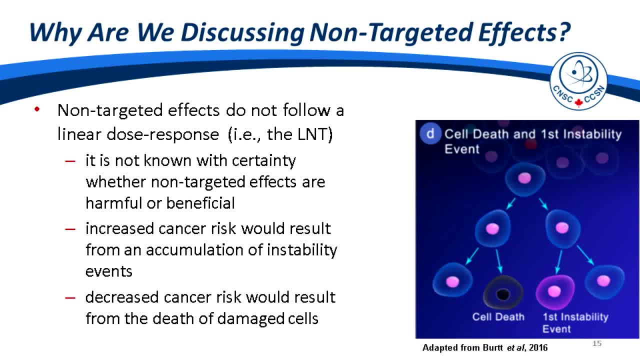 On the other hand, the studies concluding that non-targeted effects could increase cancer risk are observing an accumulation of genomic instability shown in pink as the first instability event. on this figure, An accumulation of genomic instability could then be passed onto the cell's progeny. 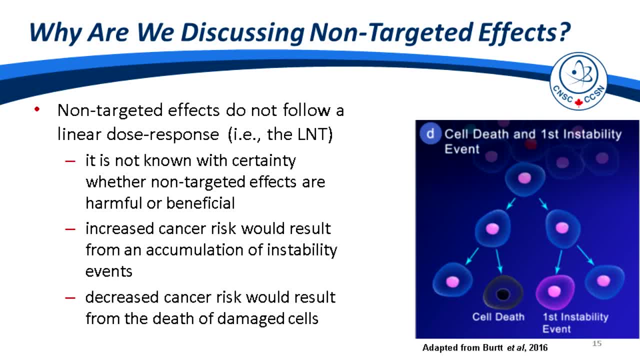 It should also be noted again that not all radiobiological effects will lead to cancer. The exact shape of the dose-response curve at low and very low doses is not known, and more research is needed to better define the mechanisms of non-targeted effects in plausible 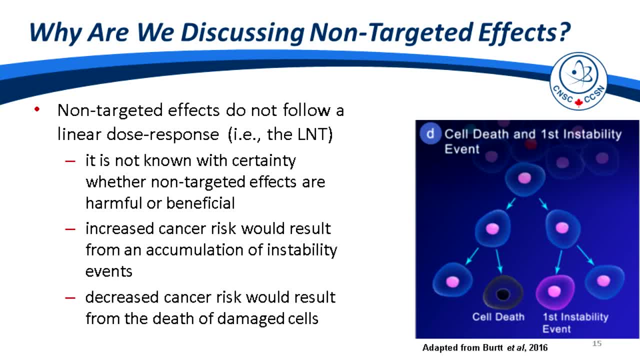 scenarios for typical human exposures. UNSCEAR has identified the need to integrate radiobiological and epidemiological research to enhance the understanding of radiation-induced health effects and associated inferred risks related to the induction of cancer, non-cancer effects and hereditary diseases. 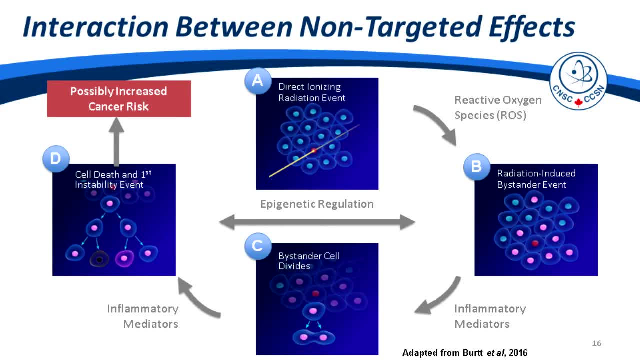 The reason why this presentation does not solely focus on the bystander effect and includes genomic instability is because there's new scientific evidence that supports the hypothesis that these two non-targeted effects interact with one another and together may facilitate cancer development, As shown on this slide, which we will go through in a clockwise manner. 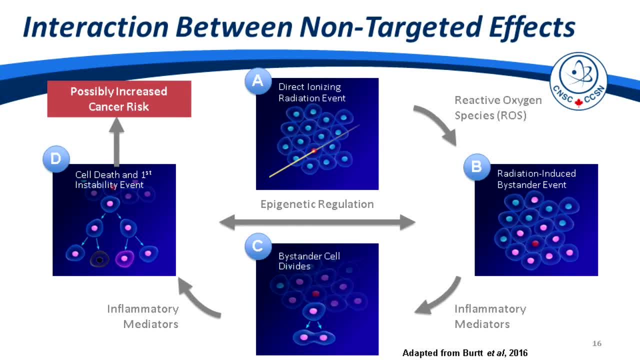 At the top in frame A, you can see a cell nucleus being directly hit by radiation, shown by a red nucleus. On the right in frame B, healthy blue nuclei have turned pink to show that they have received damage signals from the red nucleus. 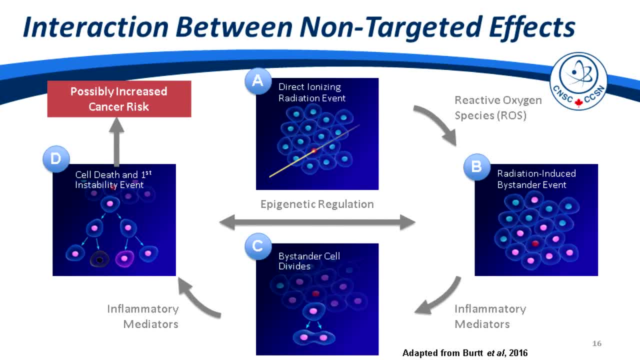 Reactive oxygen species are considered to be one of the main molecules in the chain of events That leads to the propagation of the bystander effect. If one of the affected bystander cells undergoes cell division, as shown on the bottom in frame C, inflammatory mediators could impede DNA repair or cause the cell cycle not to 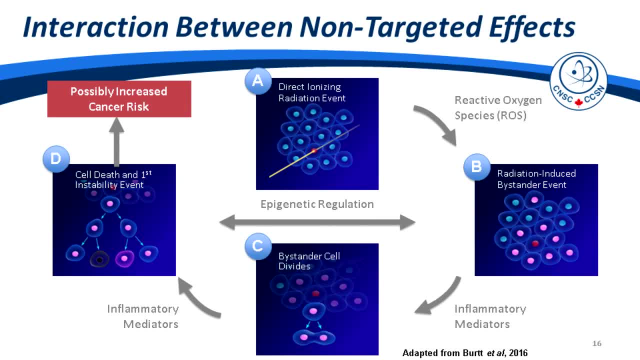 be completed properly, resulting in genomic instability. In other words, the bystander effect can induce genomic instability, as shown on the left in frame D. A possible outcome from frame D is a possible increased cancer rate. The bystander effect is a positive feedback loop between frames D and B, where bystander 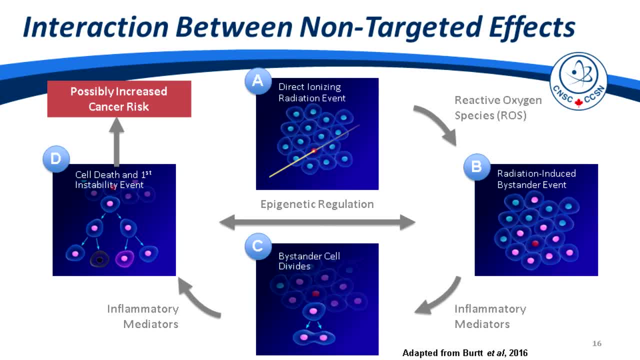 events can cause more genomic instability, or vice versa, where genomic instability is causing more bystander events, all of which have the potential to facilitate cancer development. Bear in mind that, as mentioned previously, throughout these processes, other processes, such as repair, are stopping cells from becoming carcinogenic. 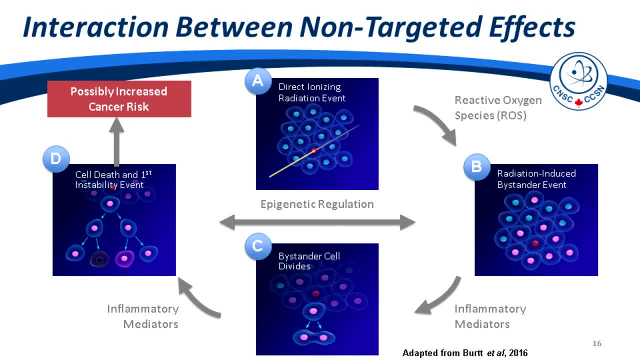 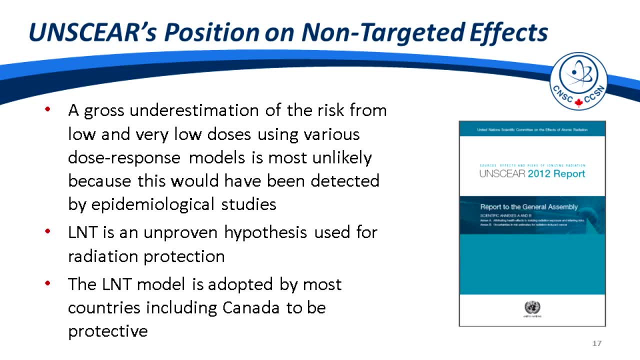 This figure is taken from a recent paper published by CNSC staff in the Journal of Radiological Protection. According to the United Nations Scientific Committee on the Effects of Atomic Radiation, the extent to which the bystander effect can modify cancer development is not known. nor. 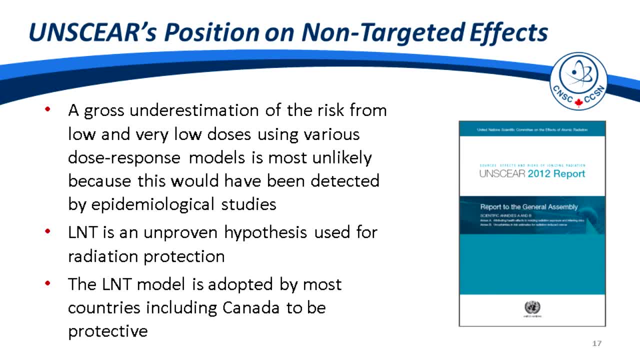 has it been established with any certainty whether these effects increase cancer risk by generating more DNA damage in neighbouring cells. This figure is taken from a recent paper published by CNSC staff in the Journal of Radiological Protection. The bystander effect is a positive feedback loop between frames D is a possible decrease. 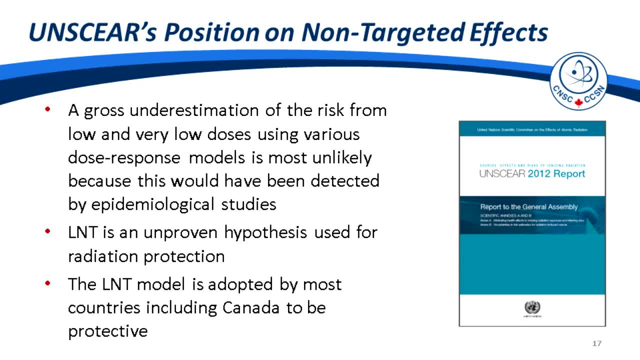 in cancer development, all of which has the potential to facilitate cancer development. The bystander effect is that the bystander effects are more likely to improve cancer development or decrease cancer risk by defective cells undergoing apoptosis and therefore stopping the perpetuation of DNA damage. 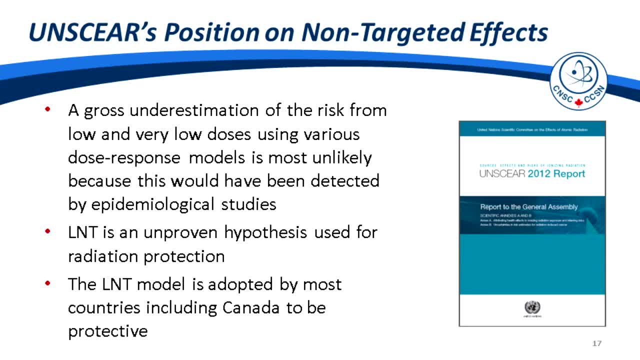 Since the publication of this report in 2012,, studies have been published in support of both of these hypotheses. UnSCIR concluded that a gross underestimation of the risk from low and very low doses using maintains their view that the LNT is an unproven hypothesis, but recognizes the need for a pragmatic 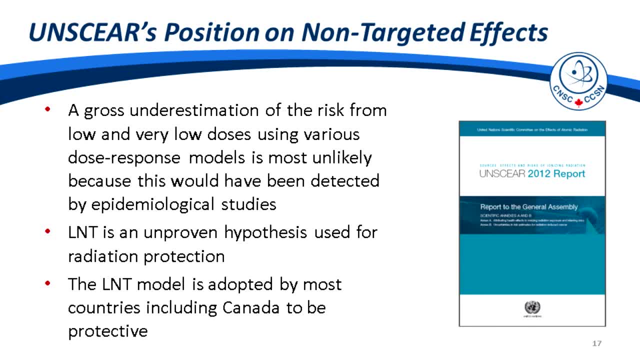 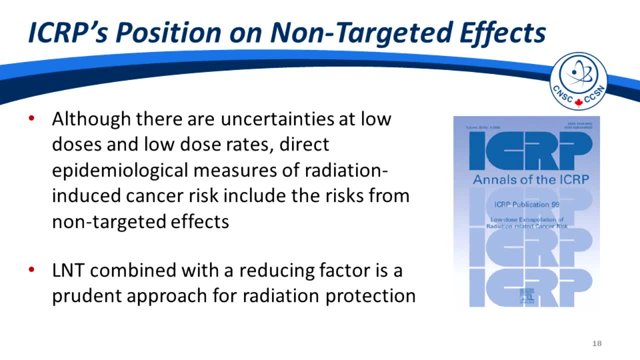 tool for radiation protection purposes. Most countries, including Canada, have adopted the LNT model for radiation protection purposes. Similarly, the International Commission on Radiological Protection is of the opinion that, although there are uncertainties at low doses and low dose rates, direct epidemiological 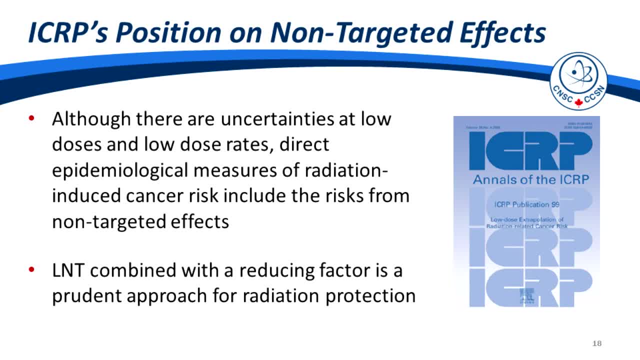 measures of radiation-induced cancer risk include the risk from all non-targeted effects. Of note in ICRP Publication 99,. the ICRPs state that, due to uncertainties in the low dose region, extrapolation from high dose effects for low dose exposures may not be. 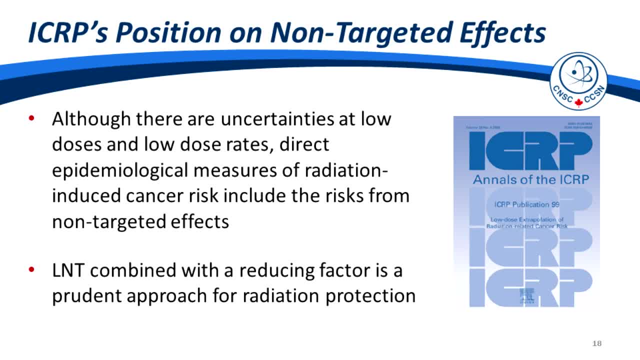 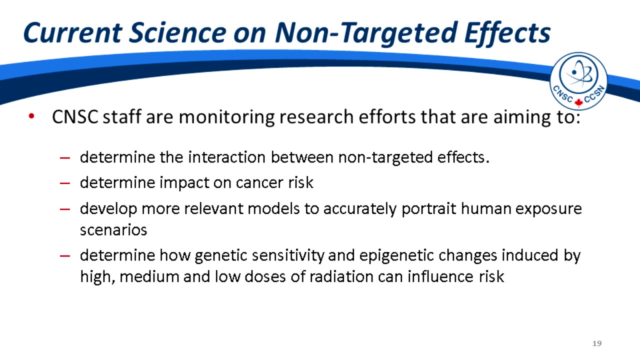 justified in all circumstances. The ICRP conclude that the LNT combined with the reduction factor is a prudent approach for radiation protection. A reduction factor accounts for the higher biological effectiveness of high doses at inducing damage. when predicting damage due to low doses from simple extrapolation. 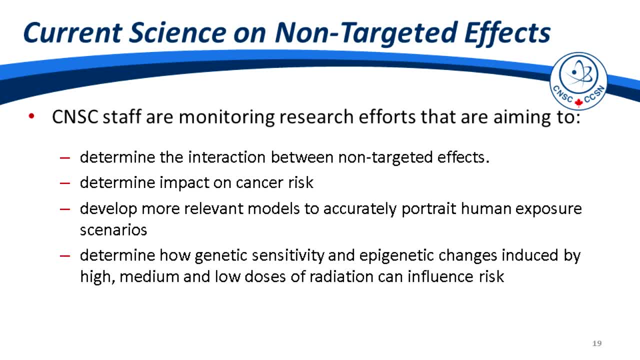 With the discovery of bystander effects and genomic instability, largely occurring in 1992, much work has been done to define the determining characteristics of these non-targeted effects. Current research efforts are aiming to determine to what extent different types of non-targeted effects interact with one another. 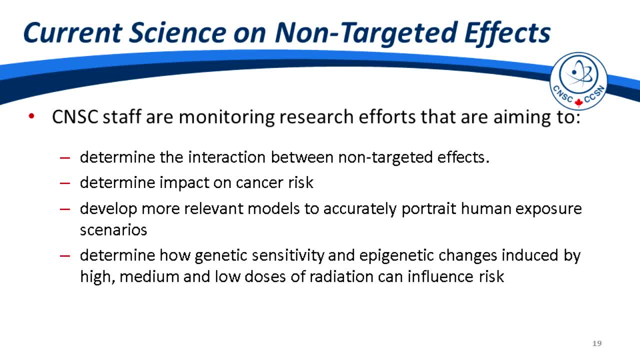 Determine whether non-targeted effects increase or decrease cancer risk. Develop more relevant in vivo models and 3D tissue models to accurately portray human exposure scenarios. Determine how genetic sensitivity and epigenetic changes induced by high, medium and low doses of radiation can influence risk. 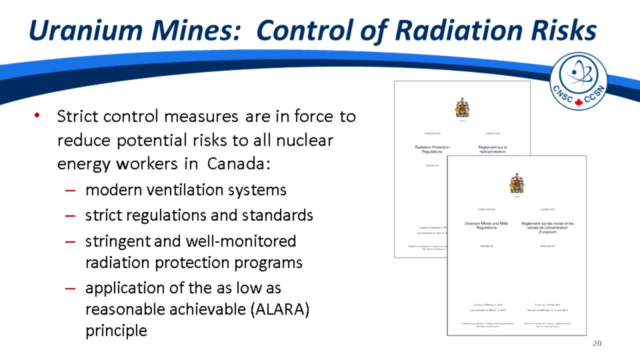 Among many other important areas of research. Slide 10. Slide 11.. Slide 12.. Slide 13.. Slide 14.. Slide 15.. Slide 16.. Slide 17.. Slide 18. Slide 19. Slide 20.. 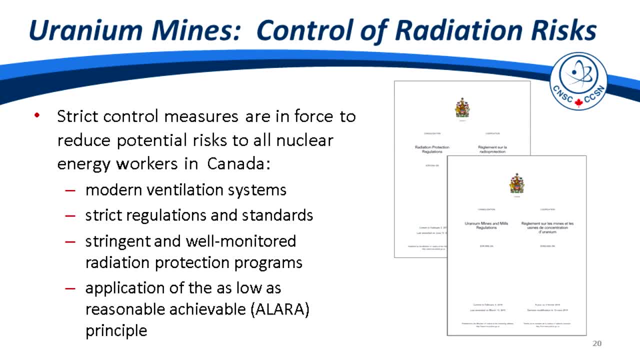 Slide 21.. Slide 22.. Slide 23.. Slide 24.. Slide 25.. Slide 26.. Slide 27.. Slide 28.. Slide 29.. Slide 30.. Slide 31.. Slide 32.. Slide 33.. 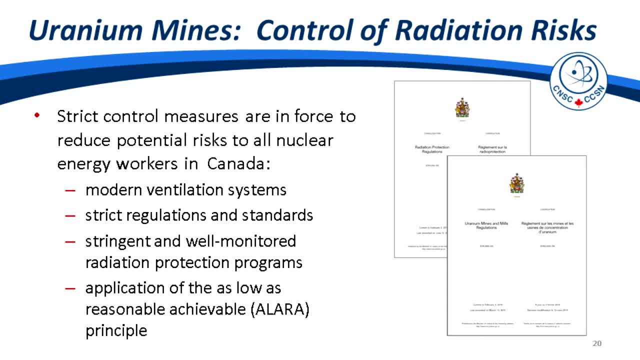 Slide 34.. Slide 35.. Slide 36.. Slide 37.. Slide 38.. Slide 39.. Slide 40.. Slide 41.. Slide 42.. Slide 45.. Slide 46.. Slide 47.. Slide 48.. 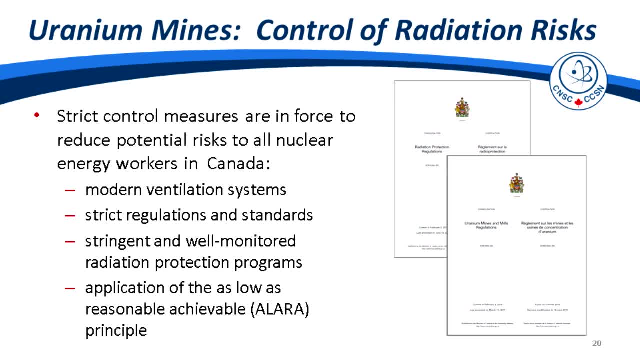 Slide 49.. Slide 50.. Slide 51.. Slide 52.. Slide 53.. Slide 54.. Slide 55.. Slide 56. Slide 56. Slide 57.. Slide 58.. Slide 59. Slide 60.. 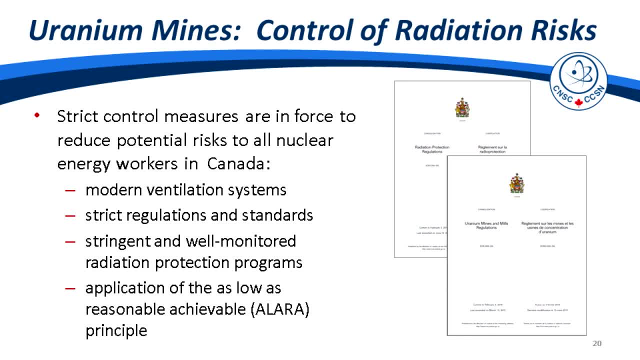 Slide 61.. Slide 62.. Slide 63.. Slide 63.. Slide 64.. Slide 65.. Slide 67.. Slide 68.. Slide 69.. Slide 70.. Slide 71.. Slide 72.. Slide 73.. 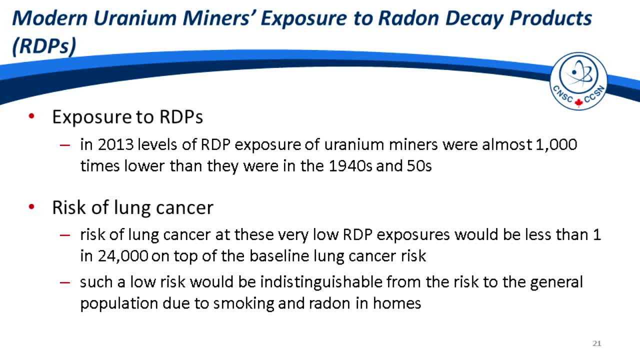 Slide 74.. Slide 75.. Slide 76.. Slide 76.. Slide 77.. Slide 78.. Slide 78.. Slide 79.. Slide 79.. Slide 80.. Slide 81.. Slide 81.. Slide 92.. 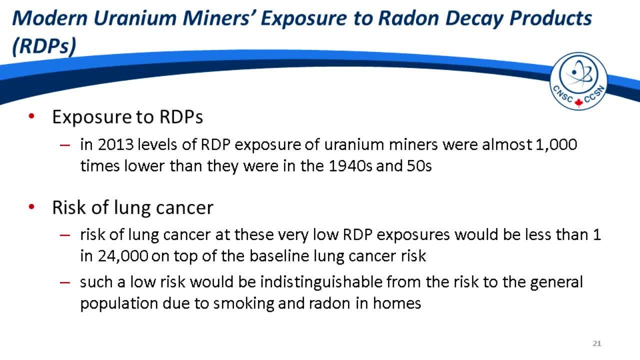 Slide 92.. Slide 93.. Slide 93. Slide 94.. Slide 94. Slide 95.. Slide 96. Slide 96. Slide 97.. Slide 97.. Slide 98. Slide 99. Slide 100.. 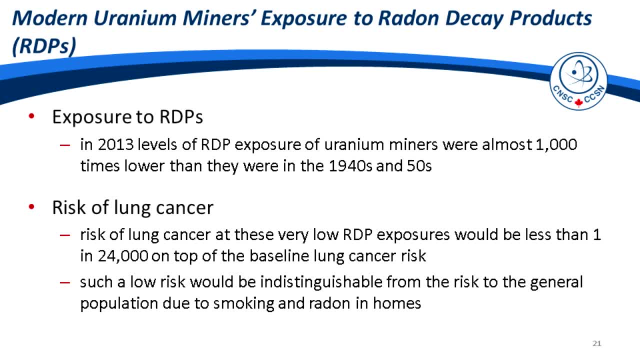 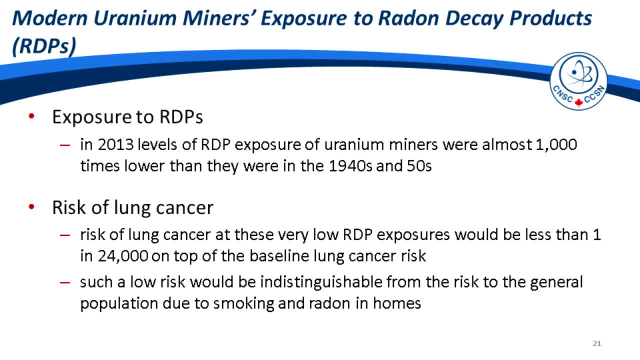 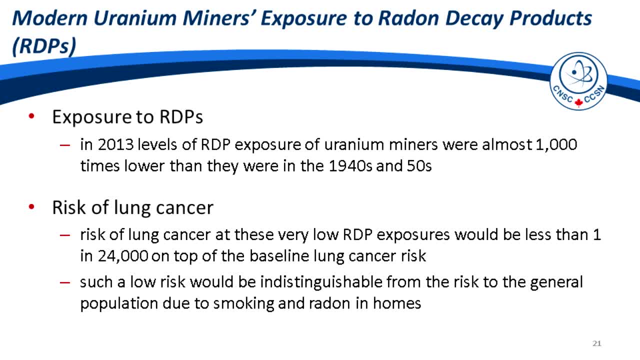 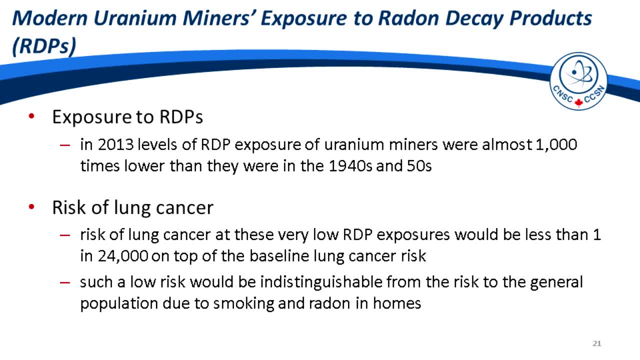 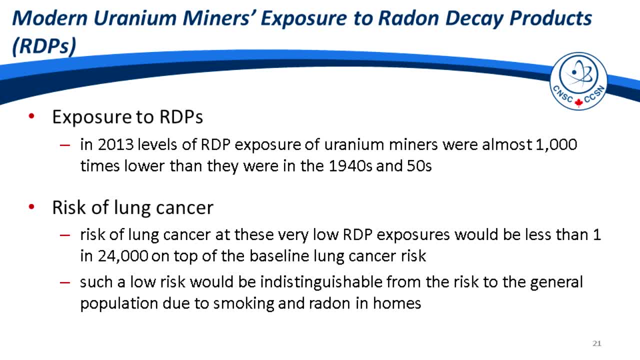